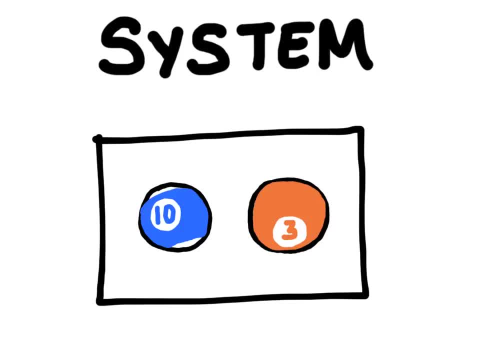 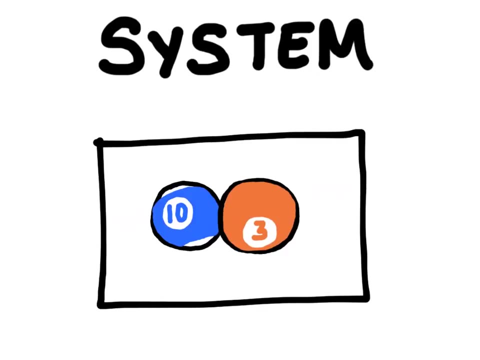 each other. this is the system, And so no forces outside of the system can interact with what's inside the system. The most common situation involving conservation momentum is going to apply when objects collide with each other, Although conservation momentum is also going to apply to objects that start together and then separate. 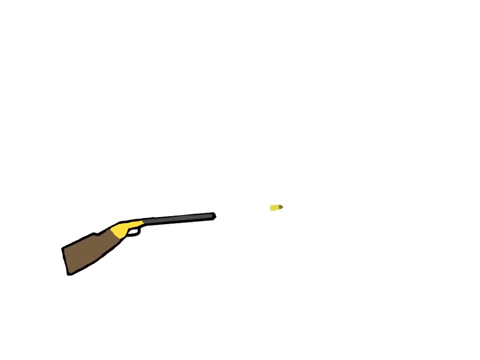 Like a bullet inside of a gun. Before the bullet is fired from the gun, the total momentum of these two objects is going to be zero. So if we take this bullet, put it right inside. Let's go ahead and prove this. Momentum is equal to m times v, where m stands for mass. 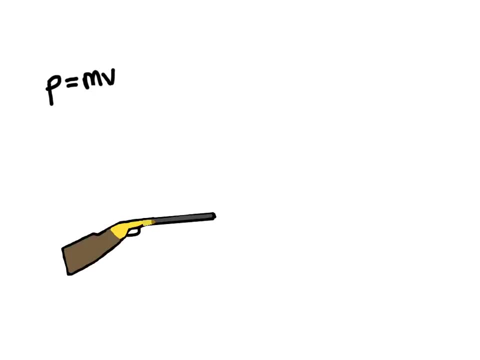 and v stands for velocity. Now we have two objects here. We have both the bullet and the gun, And their momentums together should be equal to zero. Let me prove to you that they are equal to zero Now: the mass of the bullet and the mass. 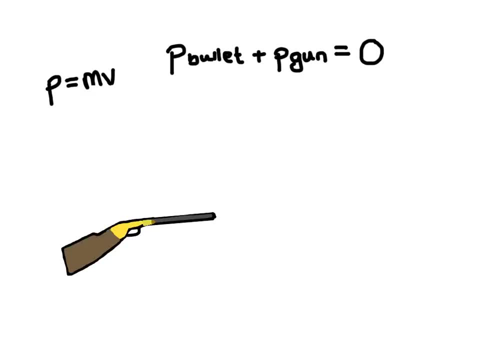 of the gun aren't really the important thing here. The important thing is the velocity or the speed of these two objects Before the bullet is fired. the speed of both of them will be zero. So if I want to prove this mathematically, I've expanded the equation here. I know that. 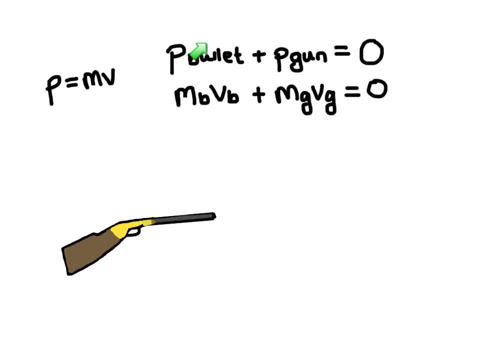 p. momentum is equal to m times v. So I've taken the momentum of the bullet and I've included the mass and the velocity. I've just indicated that this is referring to the bullet with the subscript b, And then I have mass and velocity of the gun over here. 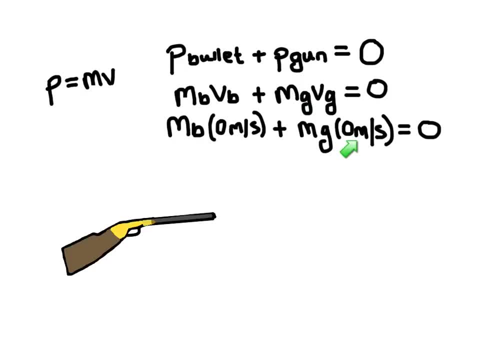 And so when I plug in the numbers here zero velocity and zero velocity, we of course get zero momentum total. Okay, so law of conservation momentum says that after the bullet is fired and leaves the gun, the total momentum of both the bullet and the gun must equal zero as well. So I'm 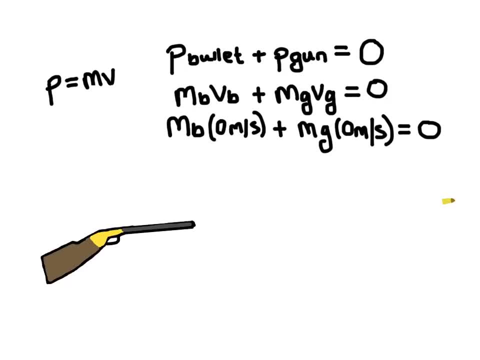 not sure how that's true. It says that the before momentum must equal the after momentum, So how could this be possible if the bullet is flying extremely quickly away from the gun? Well, let's add some masses to the bullet and the gun. 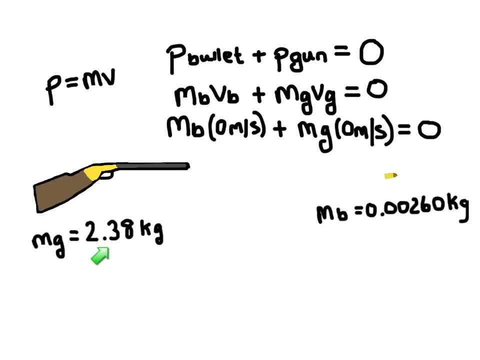 Okay, the average rifle weighs about 2.38 kg And the bullet weighs about 0.0026 kg, in other words, 2.6 grams. Now, a bullet can travel at some pretty great velocities. Let's say that our bullet is traveling at 378 meters per second. We can calculate the momentum. 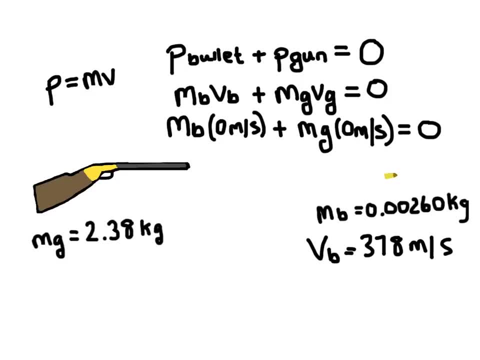 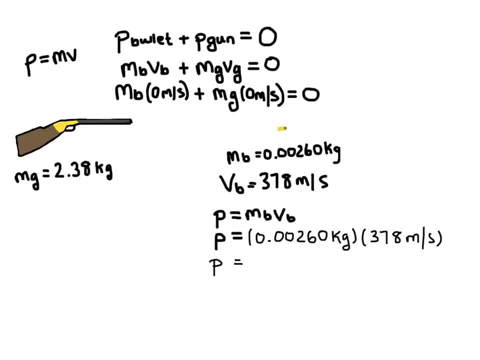 of the bullet. using the equation, P equals MV, So let's go ahead and plug in our numbers here, And so we have mass times, velocity, and we end up with momentum of 0.983 kilograms times meters per second. So that is the momentum of the bullet. Again, this is as the bullet 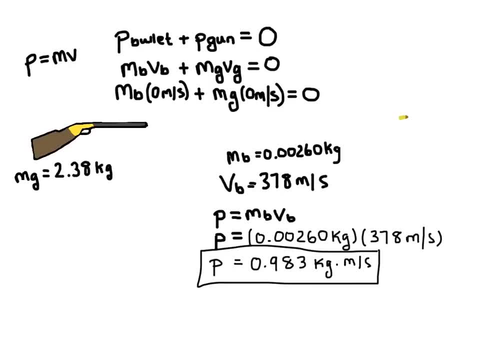 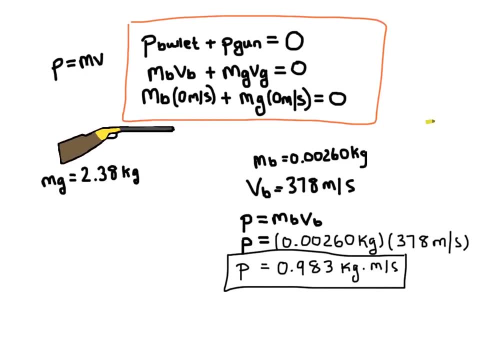 here is flying out of the gun. it's traveling with that much momentum. Now, according to the law of conservation of mass, the initial momentum, which is right here, it's 0, so we'll call this initial. it's going to have to be equal to the total momentum of the after. 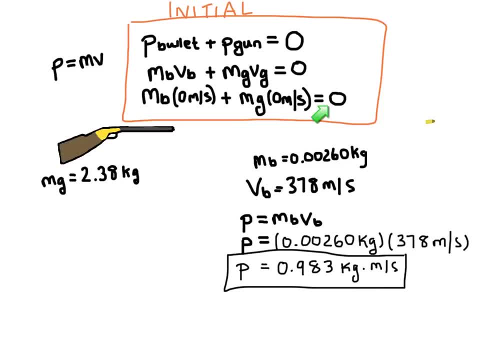 the final. So down here we're calculating the final momentum. This is the total momentum of the bullet and the gun. So that means if the bullet is traveling at positive, you can see that this is positive momentum here. 0.983, that means the momentum of the gun. 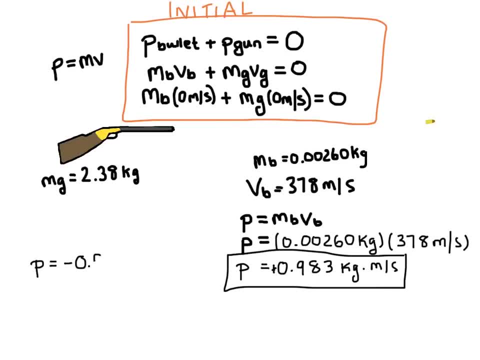 has to be negative 0.983.. Because if we add them together, they're going to equal zero, And so that would obey the law of conservation momentum. Now, when a bullet is fired from a gun, there is something called recoil, And so the bullet 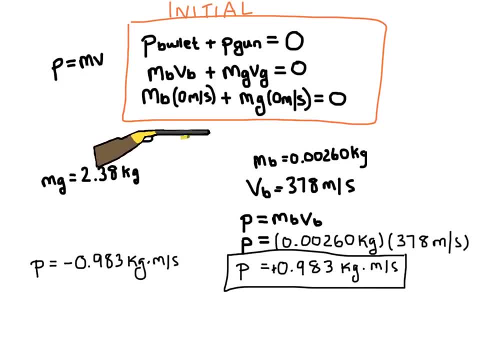 comes flying out very quickly and the gun will kind of travel backwards a little bit, And so if you're holding it and shooting it you'd feel the kick from the rifle as it bounced back. We can actually calculate how quickly the rifle would kick back The missing part that. 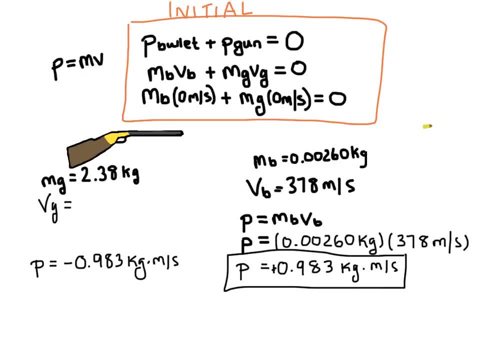 we have here is the velocity of the gun. but we can solve this because we know the mass of the gun And we know the momentum, Because the momentum is exactly equal, exactly equal to the momentum of the bullet. we should see a much smaller velocity than the.